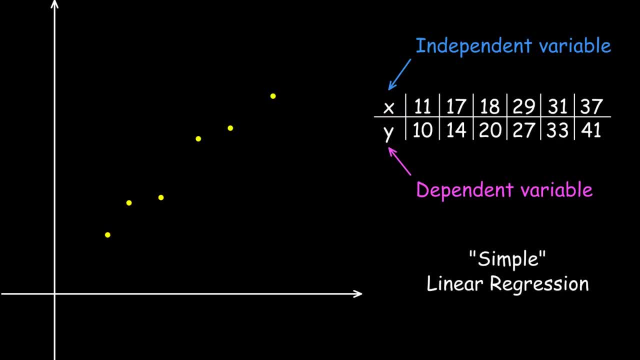 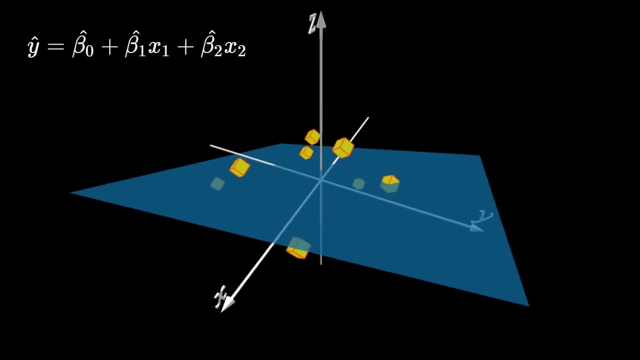 so this problem is referred to as the independent variable. A quick side note here: when we have more than one independent variable, it will be a multiple regression problem, which will be the topic of the next chapter. Anyway, we assume that the two variables have a linear relationship. 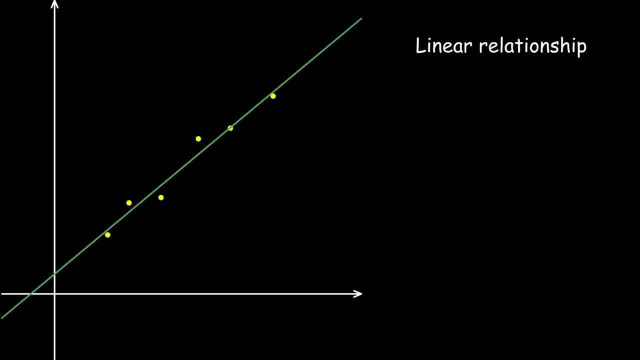 That is, as x increases, y also increases with it linearly. This linear relationship is given by the equation: y equals beta, x plus beta naught. where beta is the slope, the y-intercept, We put a hat on the beta and the beta naught. since there can be some error, 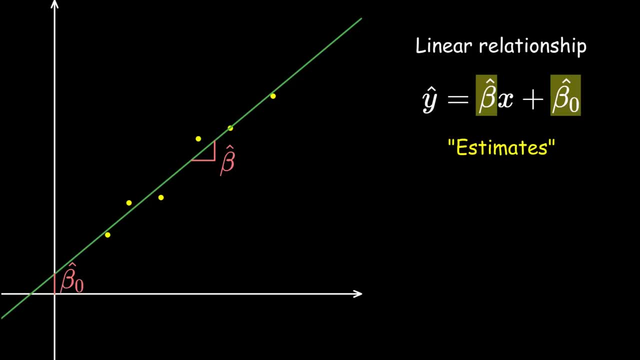 in the data and we can only give estimates of these parameters. In other words, we don't know the true values of beta and beta naught. We can only give our best guesses at them based on all the limited data we have. Likewise, we put a hat on the y, since, at any given input, 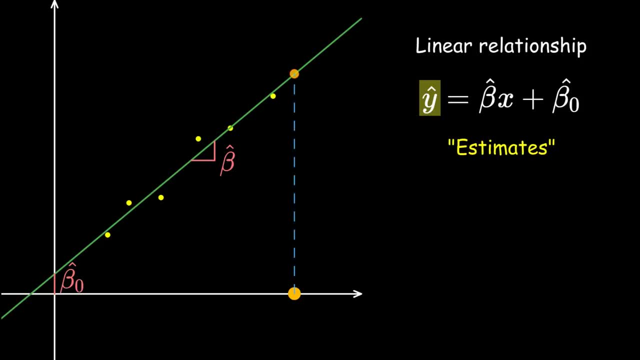 x. we are only given an estimate of the corresponding output, y, and that estimate might not be correct. The slope beta hat is calculated using this formula: Beta hat equals the sum over all x i minus x bar times y i minus y bar, divided by the sum of all x i minus x bar squared. 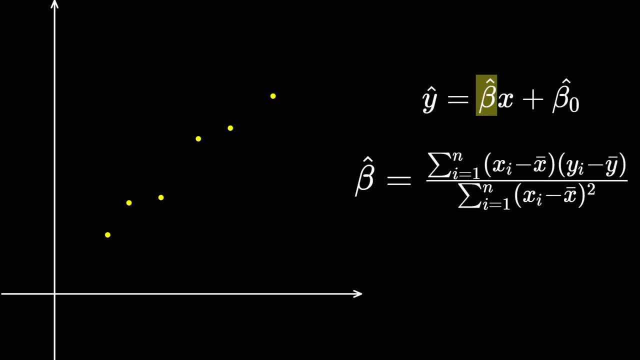 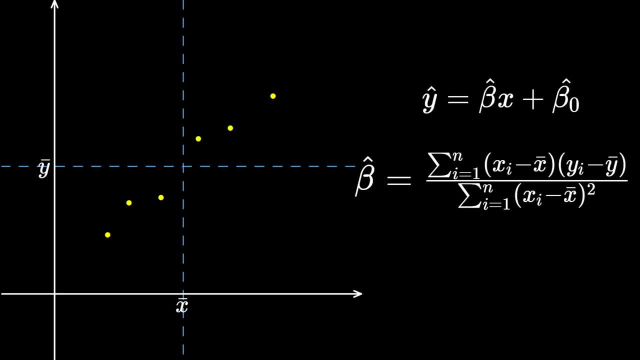 where y bar is the average value of all the y-coordinates. Let's consider this point: x1, y1.. The distance between this point and the line x equals x bar is x1 minus x bar. Likewise, its distance to the line y equals y bar is y1 minus y bar. 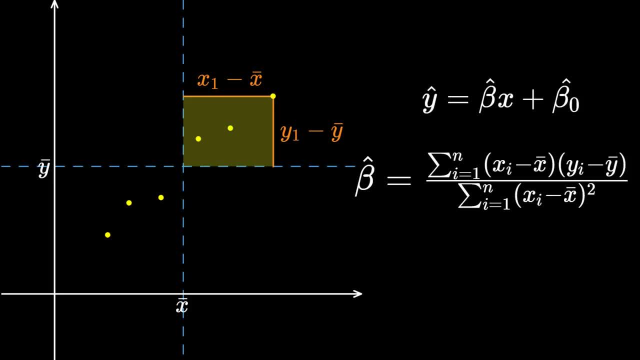 Now these four lines form a rectangle and the area of this rectangle is given by x1 minus x bar times y1 minus y bar. If we do this, for all of the data points forming rectangles with the centroid and adding up the areas, the total area of all these rectangles will be exactly equal to the numerator. 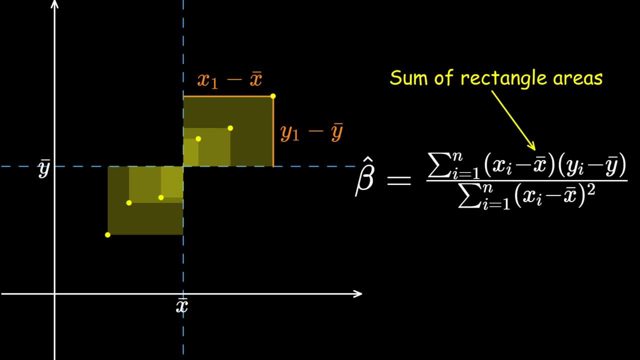 Keep this in mind for a second, because now we're going to tackle the term in the denominator. Let's first draw a line- y equals x and then project every point vertically onto that line. This way, each point will have coordinates xi, xi and the average value of all the x-coordinates. 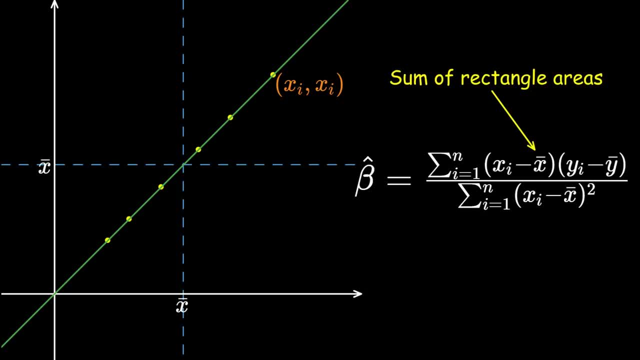 Finally, the sum of all the y-coordinates will be x bar. shown here on the line y equals x bar. Same as before. we consider all the rectangles formed with the centroid and the sum of their areas, Except this time, these shapes are not only rectangles. 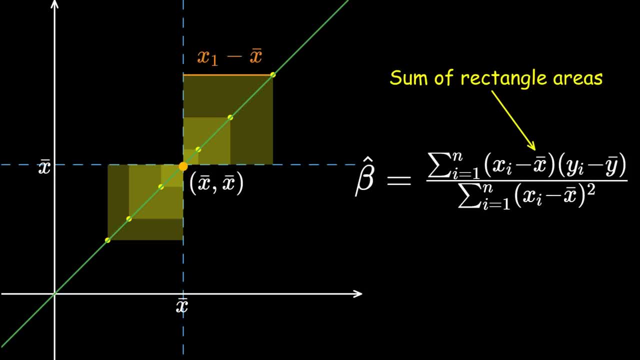 but they're also squares with side lengths xi minus x bar. The sum of their areas is equal to the denominator, the sum of all xi minus x bar squared. Indeed, we see that beta hat is given by x bar. This means that a consistivity made from a Lararoad- add economic term like cleft, at the next operation of axis, such as: skeptical behaved Marcus, ev 84 squared, đây là xa xi ra, xi-x bar square. sincerely, bets say that what we're researching is the penetration of all the yạn and x bar in all the be close to the linear coordinates of dash y diamonds. 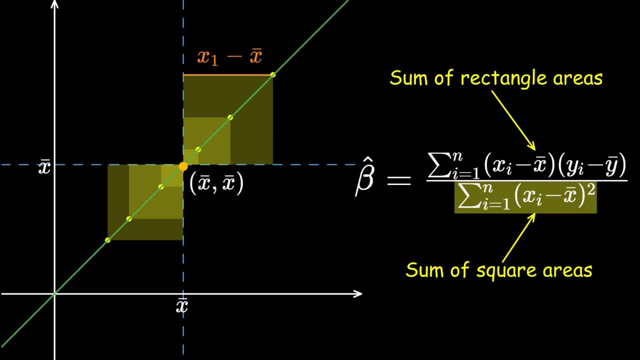 see that beta hat is given by the ratio between the sum of rectangle areas and the sum of square areas. Isn't that cool. If we restore the points to their original positions, notice that the sum of rectangle areas is a bit smaller than the sum of all the square areas. This 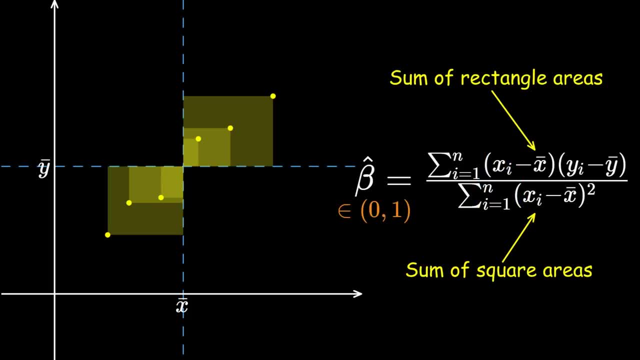 means that their ratio, which gives beta hat, is a number between 0 and 1.. Visually we see that the slope of the regression line is rather flat. In contrast, if the y-coordinates of the points are more spread out, then the rectangle areas will be greater than the square. 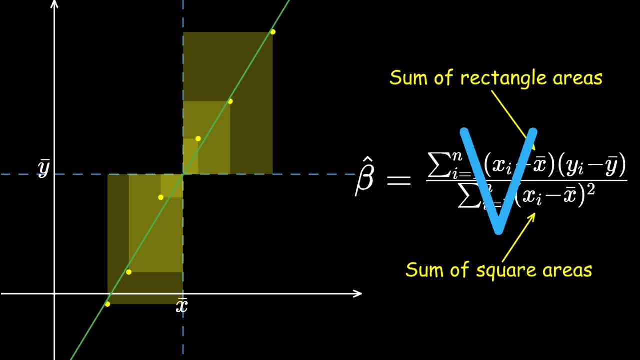 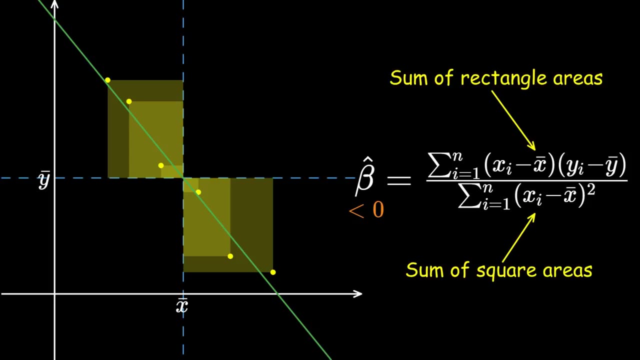 areas. As a result, beta hat is greater than 1, and the regression line gets steeper. Also, it is possible for the regression line to have a downward slope, which implies that beta hat is negative. If the points of the regression line are more spread out than the square areas, then the 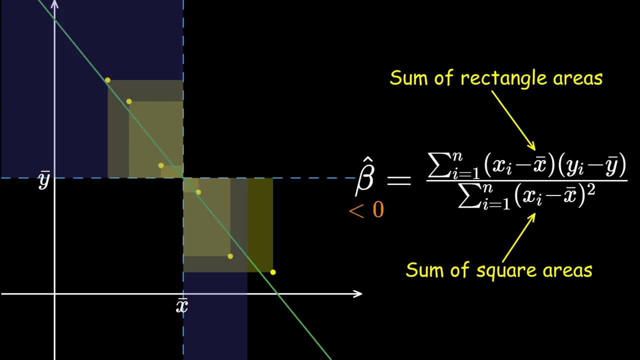 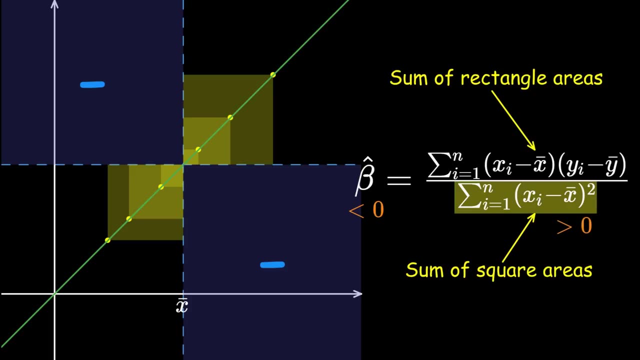 points are living in the top-left quadrant of the center point or the bottom-right quadrant, then you will be adding up the quote-unquote negative areas of the rectangles. Of course, when you divide by the sum of square areas, that value will always be positive as the